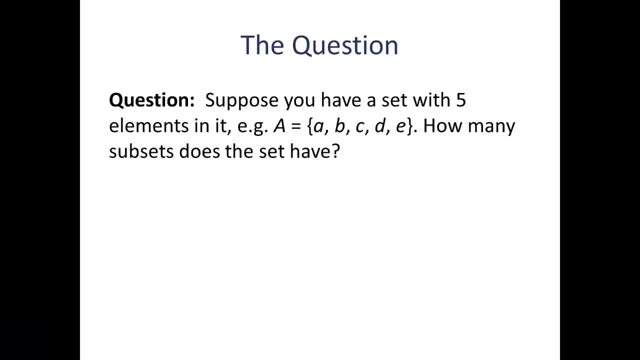 The question asked here- how many subsets does a set have- is actually an important question from set theory that we can answer using our combinatorics methods. In this case, we're looking specifically at a set with five elements- A, B, C, D and E- and asking the question: how many subsets does it have? 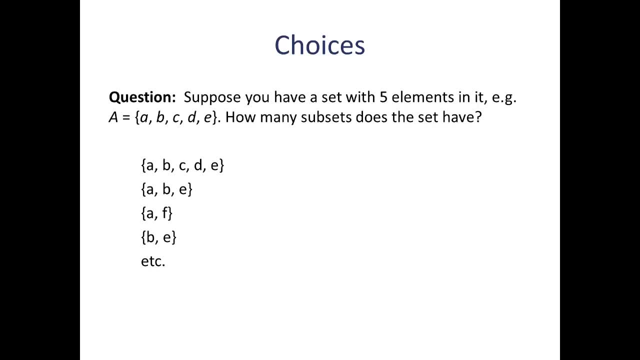 What makes this question complicated is that we have to count subsets of a variety of sizes. For example, we have to count the subsets with three elements, like A, B and E, subsets with two elements, like A and F, etc. 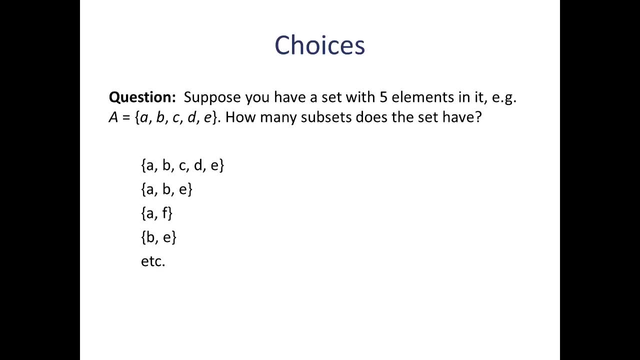 So, to answer this, we're going to have to kind of be a little more creative in our thinking. Here's how we're going to approach it. When I'm choosing a subset, the choice I have to look at for each of the five elements is: is this element in the subset or isn't it? 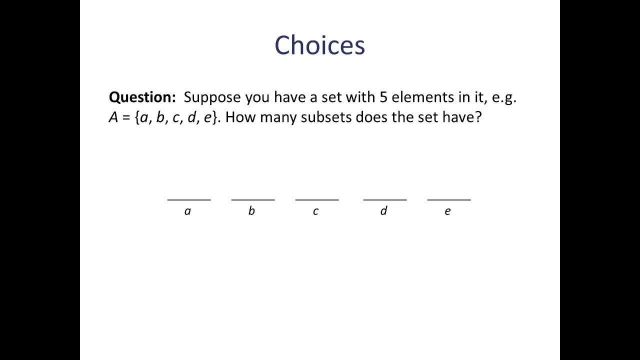 So to do that, I'm going to start with five lines, five spaces or blanks, one for each element. Now, for each element, I have two possible choices: Either that element is in the subset or it isn't in the subset. 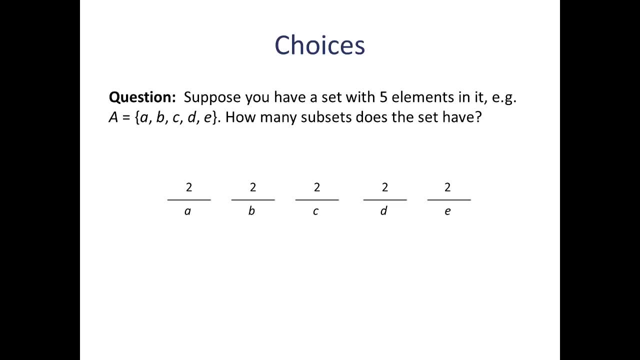 So I'm going to put a two in each of those spaces to represent those two, Two options for each one. Now, at this point, the multiplication rule applies and we can get the total number of combinations by multiplying all five of those twos together. 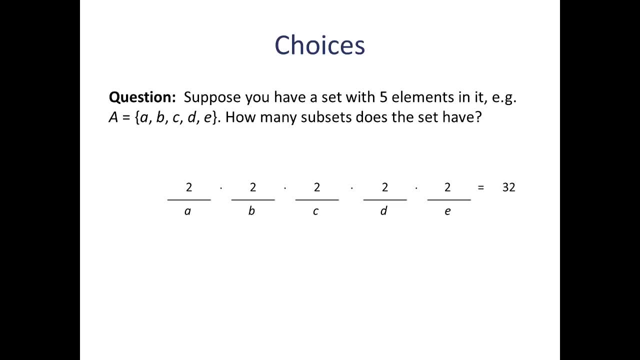